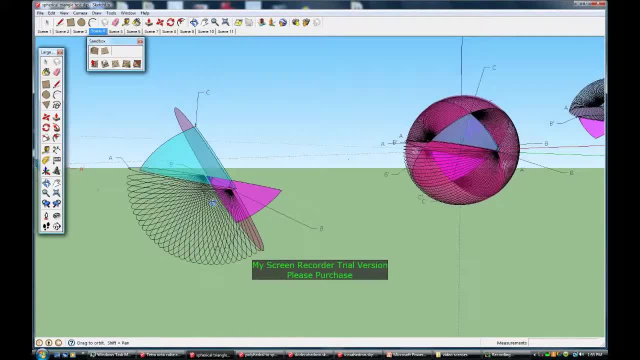 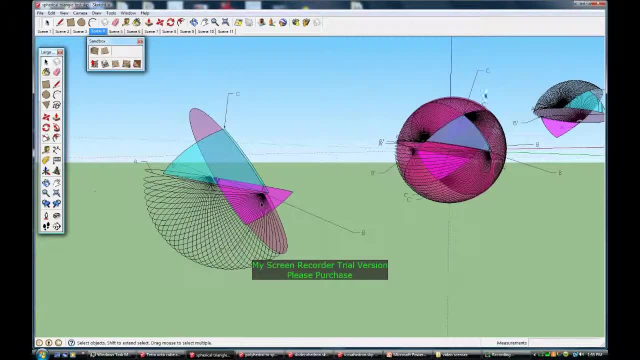 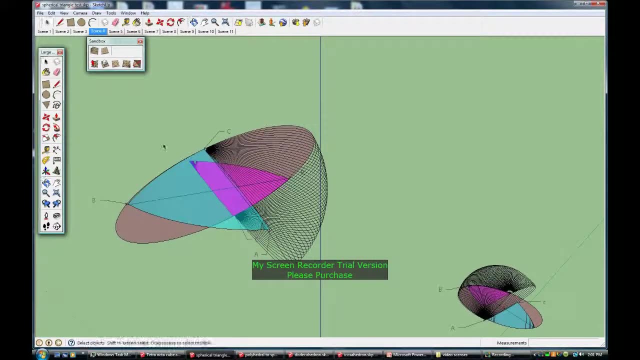 useful to draw these things in SketchUp and get a three-dimensional version of it that you can rotate around And see from different perspectives. So that's the second bianchial region And here's the third bianchial region. You continue your counterclockwise rotation around here and draw a great circle from C. 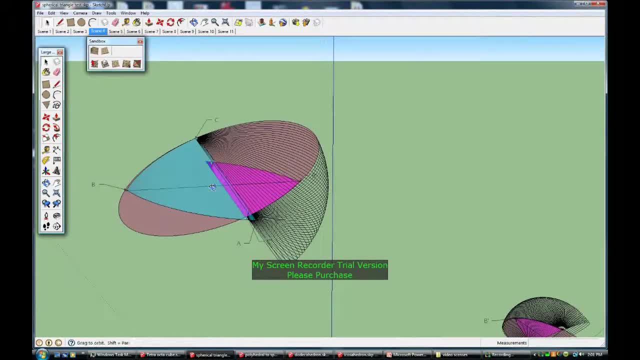 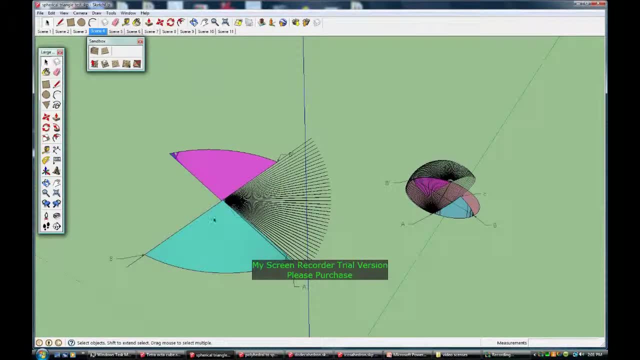 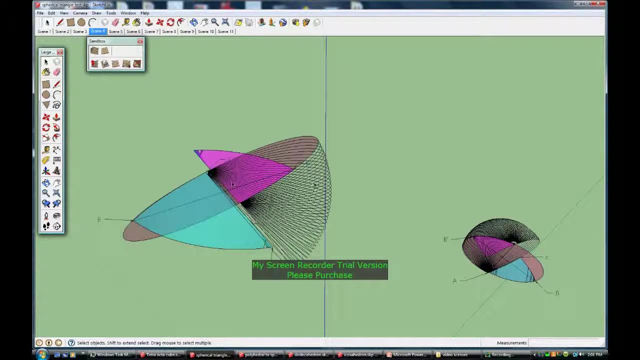 to A, around to the other side, at C prime and then back through B prime, And again the angle is just the angle, pi or 180 degrees minus the angle at B prime, And again the angle is just the angle of the radius, so it's just pi minus gamma. 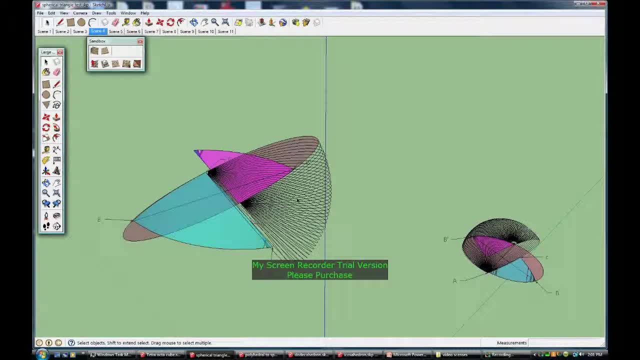 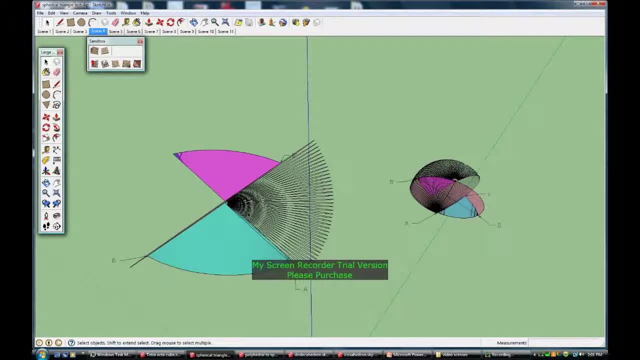 And the area of this region is just that angle: pi minus gamma times two times r squared the radius. So if this angle weren't the short angle but went all the way around, so it was two pi, it would be two times two pi, which would be four pi r squared, which is the area of 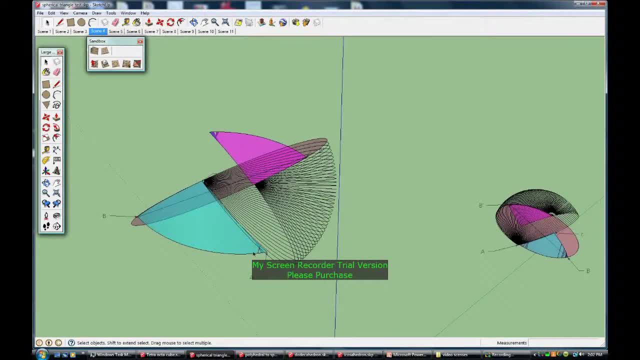 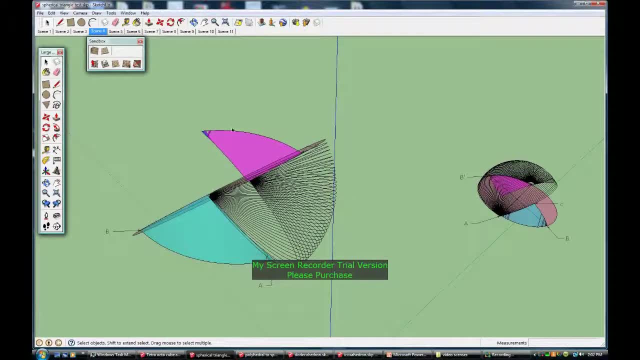 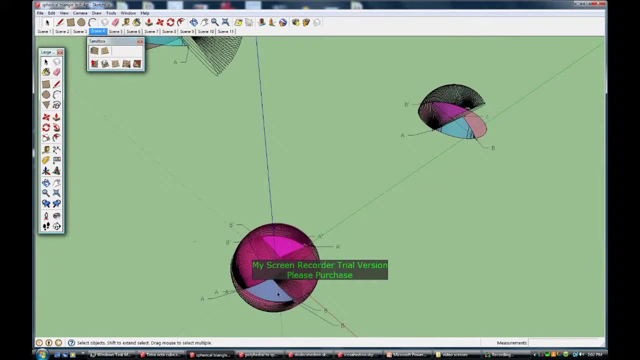 So that's the third region right there. so you see that you get three biangular regions to go with the triangle itself and the inversion triangle, And the interesting thing about that is that it covers the entire surface of the sphere. So the sum of those three biangular regions and two. 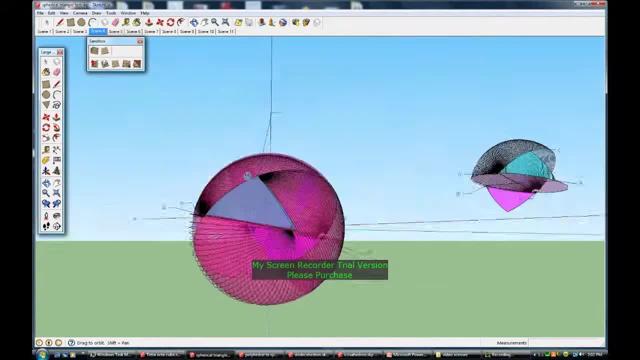 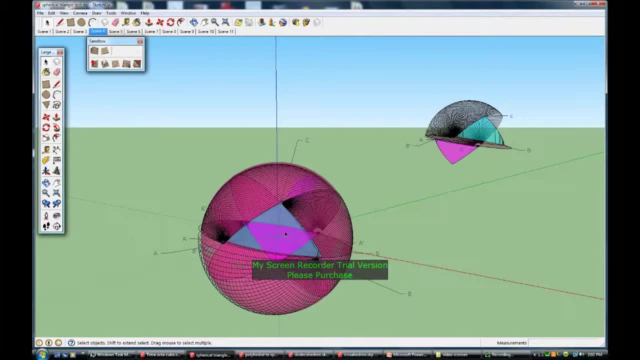 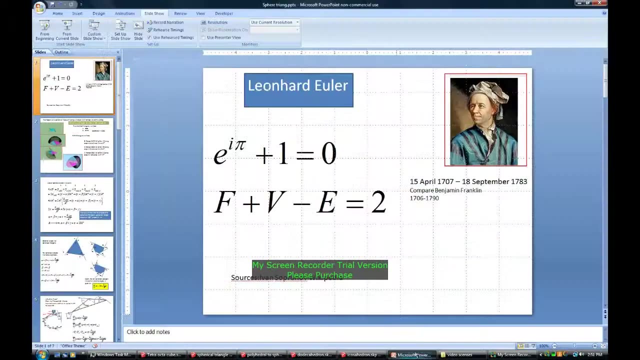 triangular regions is equal to the area of the sphere, And then you're going to use that to show relationships between the angles and the areas of the geometric figures. And let me just show that next. Alright, let's go back to Euler for a second. here And there he is. So basically we 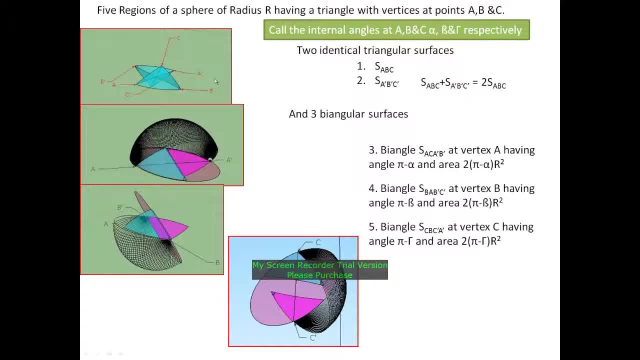 showed that we can cover the entire sphere with five regions defined by any arbitrary triangle, ABC. So we'll just use the notation S, sub ABC, the area of ABC. And then there's another one which is the inversion of S ABC on the opposite side of the sphere, called S A, prime B. 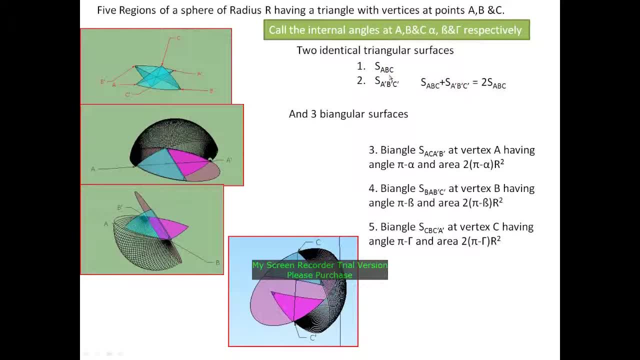 prime, C prime. Those two are equal. They're formed by the exact same angle. It's just one is the inversion of the other Through the center of the sphere. And so S ABC plus S A prime, B prime, C prime is just two times S ABC, two times the area of the triangle. That's the first part of. 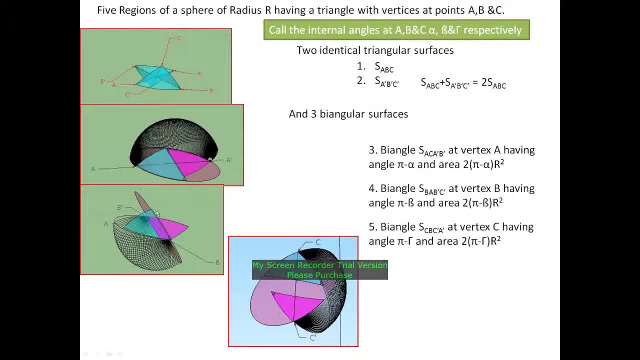 the partition, those two triangles, And then we get three biangular regions which cover the remainder of the sphere: The biangular, the biangle AC, that's the angle at A, AC, A prime, B, prime at vertex A, having angle pi minus alpha Alpha is the 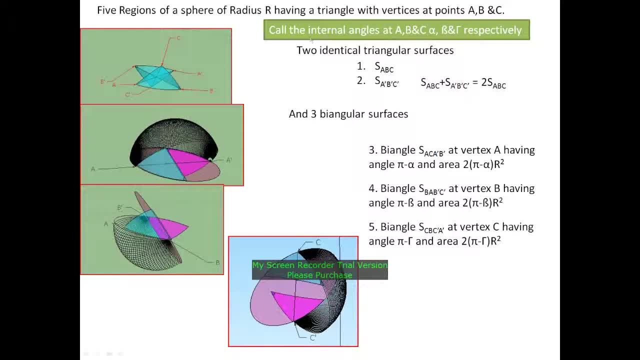 internal angle at A. So we just call the internal angles at the triangle vertices A, B and C alpha beta gamma. Sorry, sometimes I use capital gamma, Sometimes I use small gamma. A little bit inconsistent of that because of different softwares. 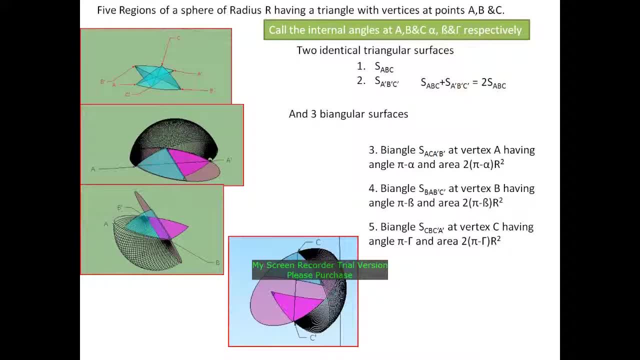 Forget it. But anyway, then there's the set, the part four, the biangle at B which just goes B A, B prime, C prime. those vertices of those points define that biangle. It has angle, pi minus beta, pi minus the internal angle at B, and an area given by two times pi minus beta times R. 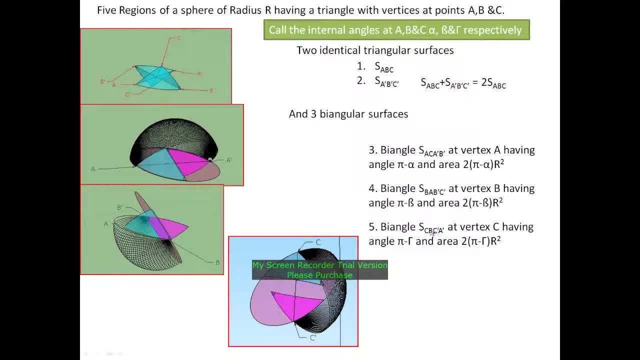 And then five: the biangle at C, S, C, B, C, prime, A prime at vertex C, having an angle pi minus gamma and an area of two times pi minus gamma, times R squared. So basically, every time you draw a triangle on the surface of a sphere, every triangle, every spherical triangle, ends up having a partition of the entire surface of the sphere in 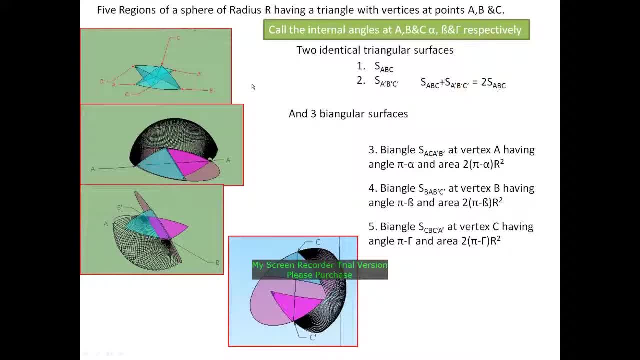 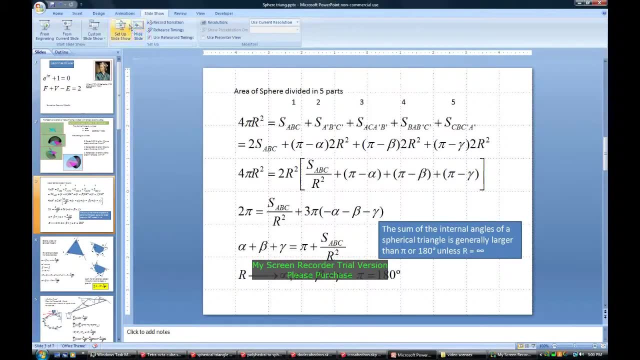 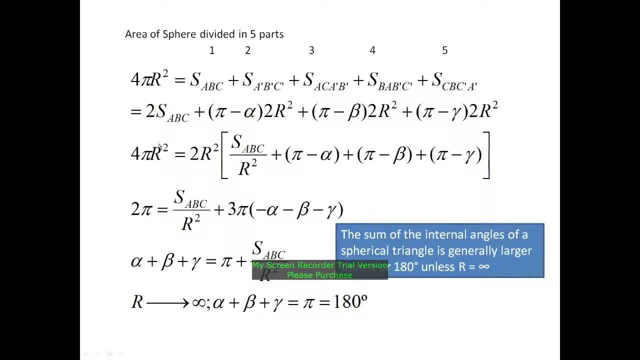 these five kinds of regions, And from that you can generate a simple equation. Okay, the next thing is to write down the whole equation- And I've got to be careful here with the equations, because the watermark, as they call it, will end up covering up my conclusion, or something. 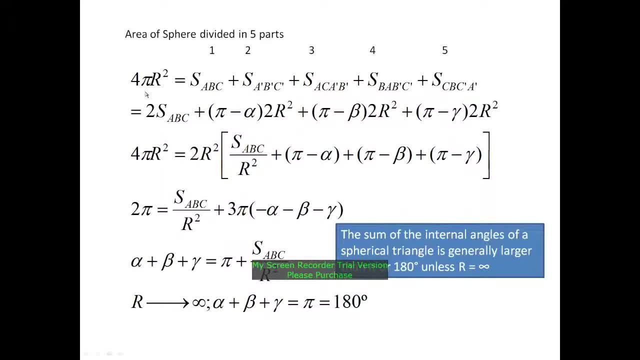 I don't know, But I know I'm okay up here at the top. So we divided into five regions And then we set that equal to the entire area of the sphere, For pi R squared is the area of the sphere for any radius R. 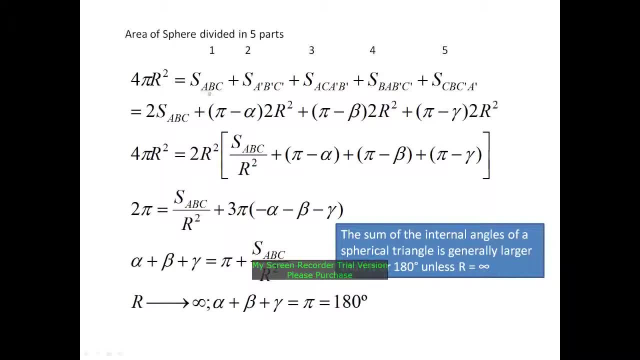 And then these are the five regions for any triangle ABC, And that can be expressed in terms of the internal angles. Because of the internal angles of those, the angles of those biancular regions are pi minus B, That's alpha, pi minus beta. 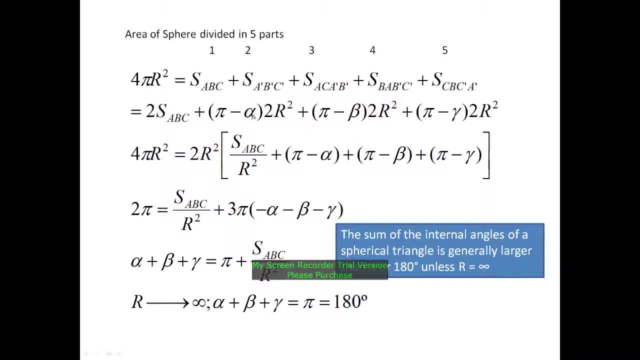 Pi minus gamma, All times two R squared to get the area of those biancular regions, And then this is two times ABC, because the area, the surface area of ABC and the surface area of A, prime, B prime, C, prime are the same. 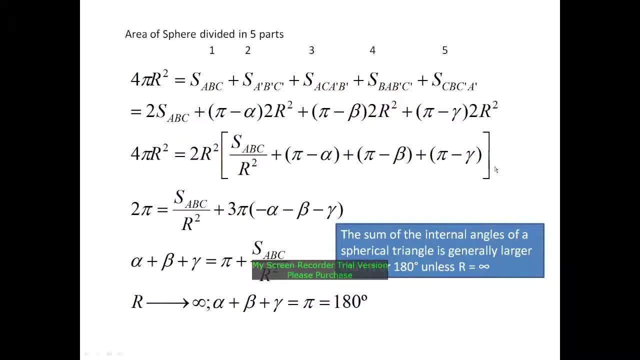 Then you can just solve this for alpha, beta and gamma- three internal angles of the triangle, And you just follow the kind of obvious algebra through here And you get the sum of the internal angles of any spherical triangle on the surface of the sphere is alpha plus beta plus gamma. 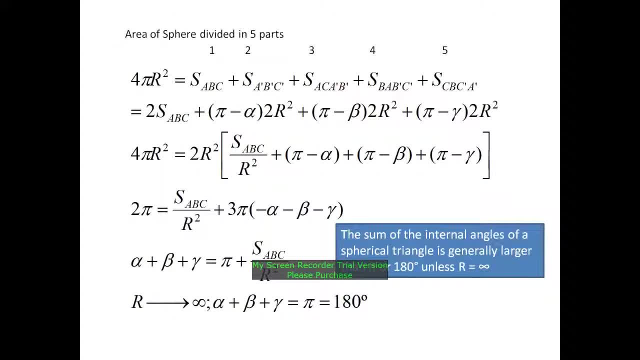 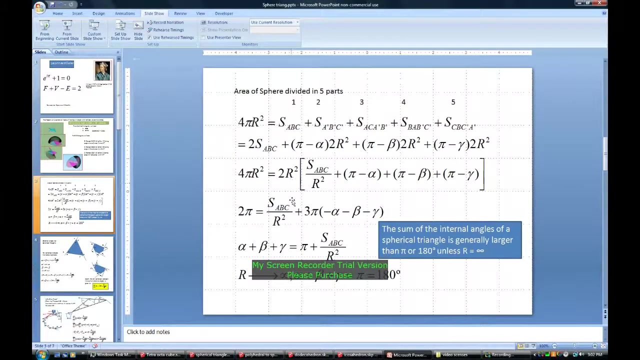 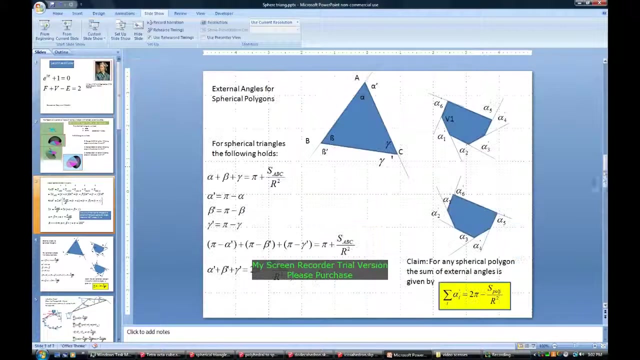 The internal angles at vertices A, B and C of any random triangle is pi or 180 degrees plus the surface area ABC of the triangle divided by R squared. So essentially what you see is that. let me just raise that up just in case it's not covered, in case it gets covered by my watermark here. 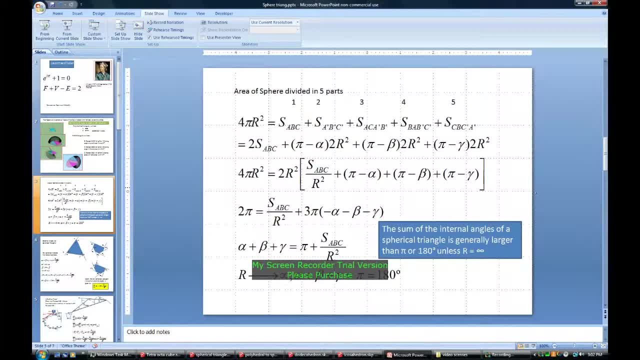 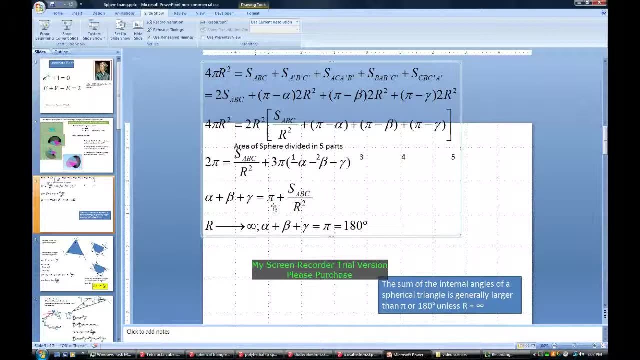 How do I do that? Let's see. Let's just bring this up here like this: Okay, The sum of the angles alpha plus beta plus gamma equals pi plus S, A, B, C over R squared. Now recall what happens if? well, let's look at what happens if R goes to infinity.